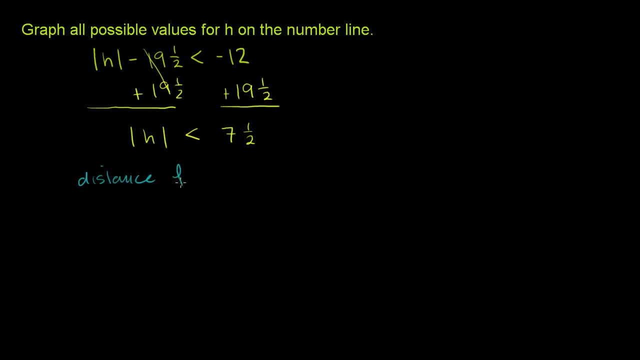 distance. The distance from h to 0 has to be less than 7 and 1 half. So what values of h are going to have? less than a distance from 7 and 1 half? Well, it could be less than 7 and 1 half and greater than 0.. 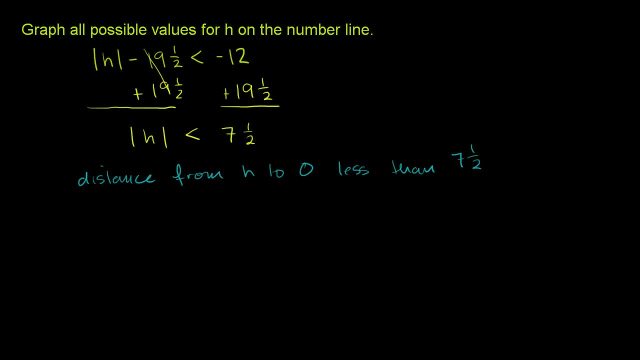 Or equal to 0. So let me put it this way. So h could be less than 7 and 1 half. But if it gets too far, negative. If it goes to negative 3, we're cool. Negative 4, negative 5,, negative 6,, negative 7,. 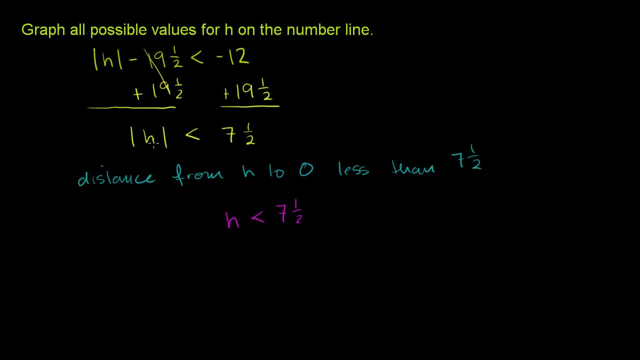 we're still cool, But then, at negative 8,, all of a sudden, the absolute value isn't going to be less than this, So it also has to be greater than negative 7 and 1 half, If you give me any number in this interval. 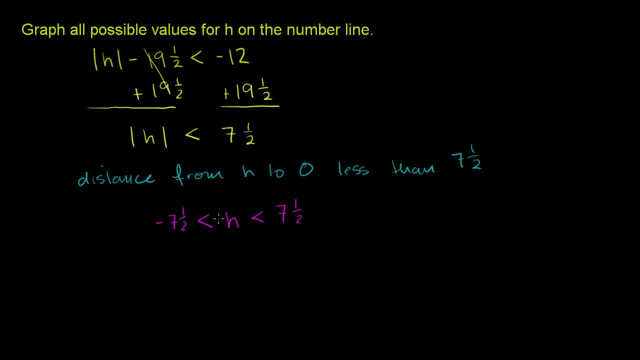 its absolute value is going to be less than 7 and 1 half. Because all of these numbers are less than 7 and 1 half away from 0.. Let me draw it on the number line, which they want us to do anyway. 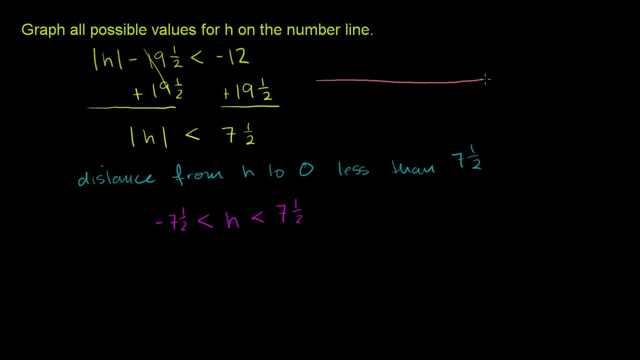 So if this is the number line right there, that is 0.. And let me draw some points. Let's say that this is 7, that is 8, that is negative 7, that is negative 8.. What numbers are less than 7 and 1 half away from 0?? 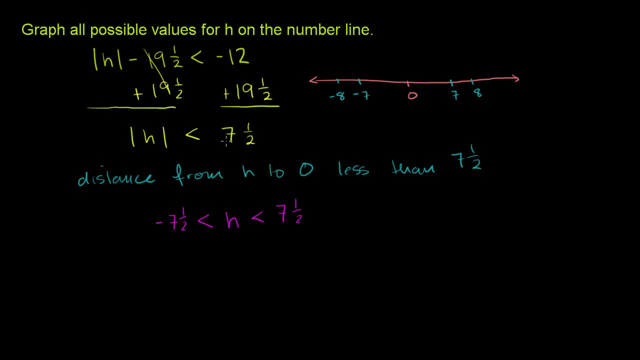 Well, you have everything all the way up to 7 and 1 half is exactly 7 and 1 half away, So you can't count that. So 7 and 1 half, you'll put a circle around it. Same thing true for negative 7 and 1 half. 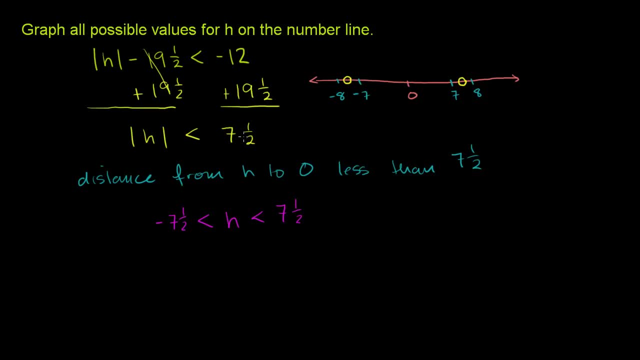 The absolute value. it's exactly 7 and 1 half away, But we have to be less than 7 and 1 half away, So neither of those points are going to be included: Positive: 7 and 1 half or negative: 7 and 1 half. 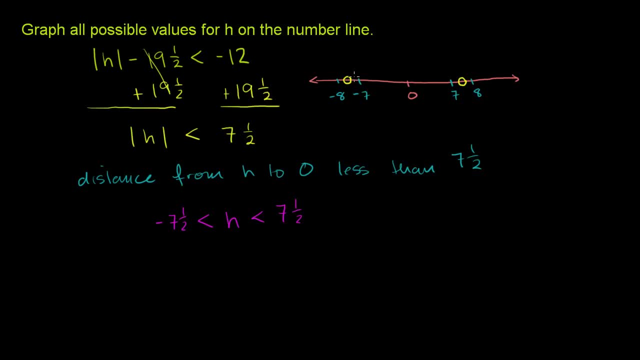 Now everything in between is less than 7 and 1 half away from 0. So everything else counts. Everything outside of it is clearly more than 7 and 1 half away from 0. And we're done.